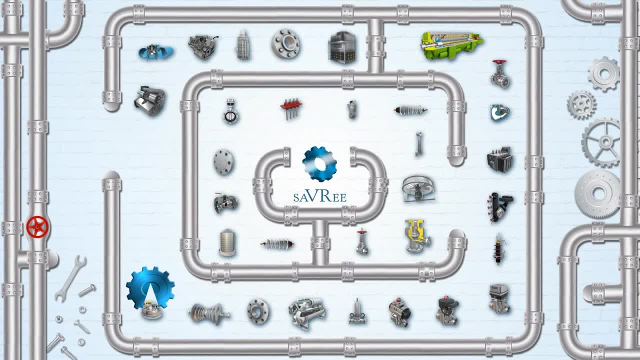 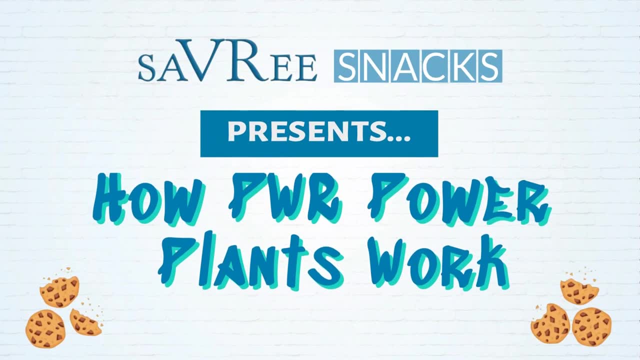 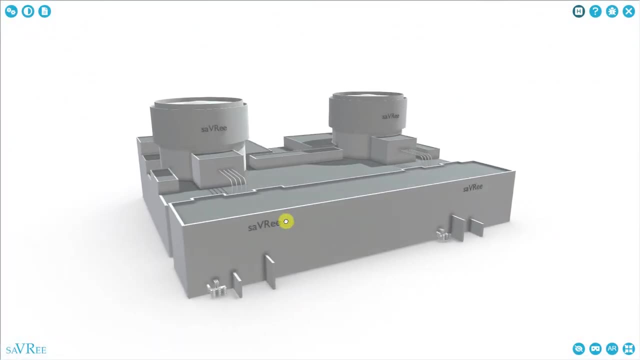 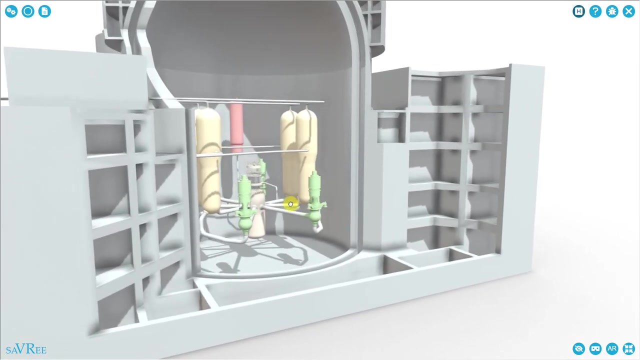 and I'll show you how it works. Here is our pressurized water reactor nuclear power plant. I'll take a cross section. I can show you some of the main parts. We've got our nuclear side. That's actually everything over here. 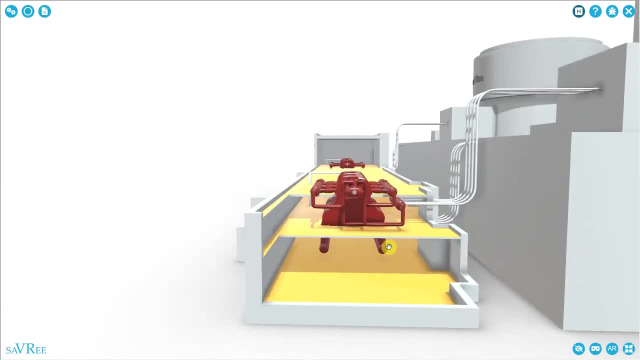 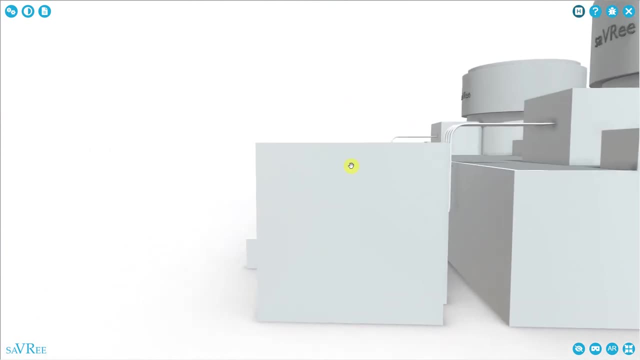 and then we've got our conventional side, which is everything over here. So the one building over here would be our nuclear side and the one building over here would be our conventional side. The conventional side's called conventional because we deliver steam to steam turbines. 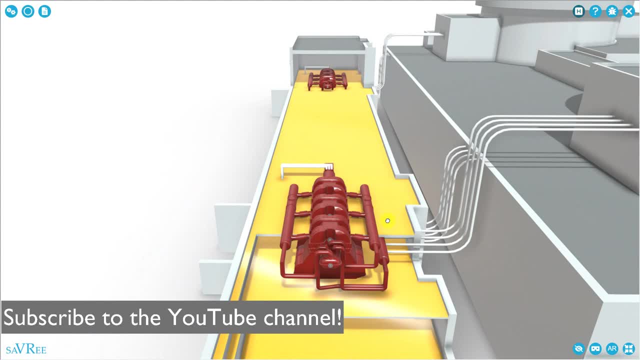 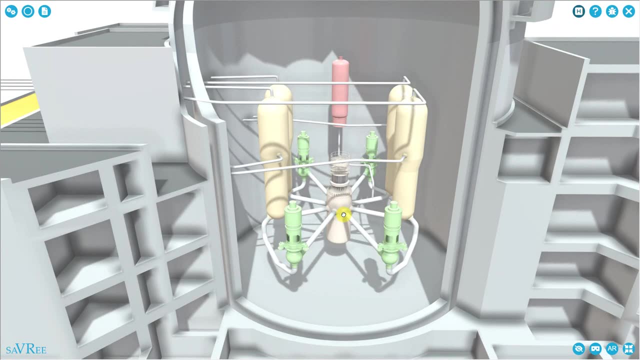 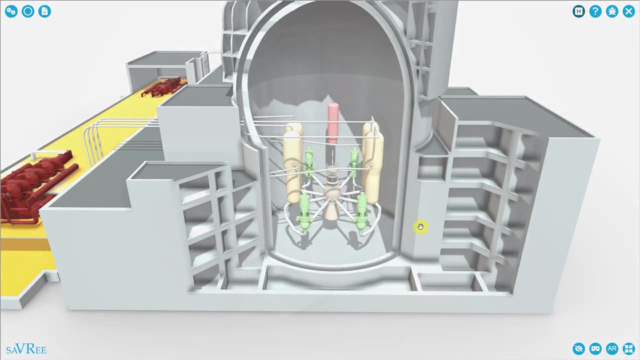 and those steam turbines then generate electricity via a generator On the nuclear side. this is- I suppose you could dub it- unconventional. It's slightly different. It acts as our heat source. If we were to replace this entire nuclear building with a coal-fired boiler. 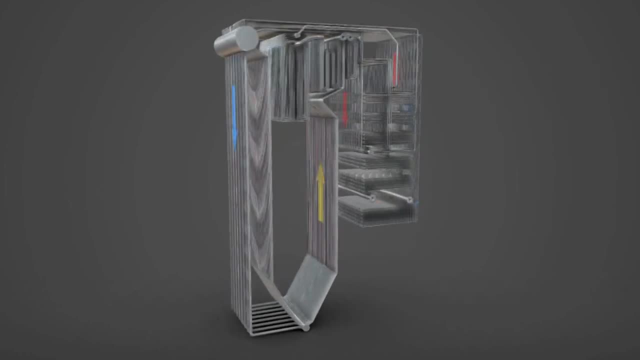 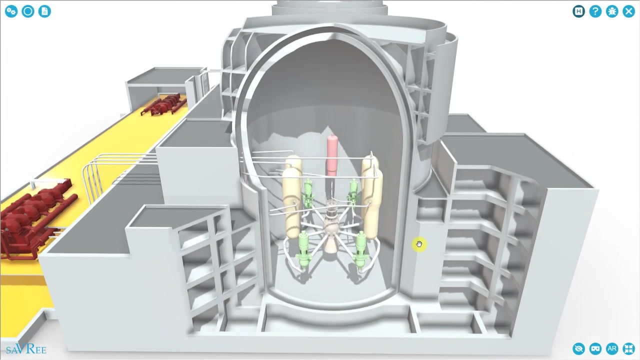 a gas-fired boiler or anything else that we could use as a heat source, then we would have the same effect: We would use it all to generate steam. So that's exactly what's happening on the nuclear side of our power plant: We're generating heat and using it to turn water into steam. 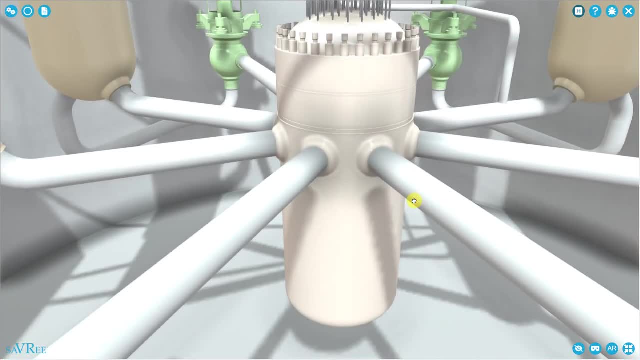 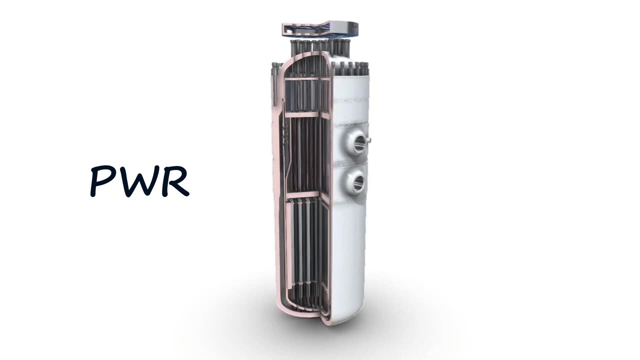 To generate the heat, we use a nuclear reactor. This one is a pressurized water reactor, PWR. The other type that you're quite likely to see if you work in the nuclear engineering industry is a boiling water reactor, BWR. 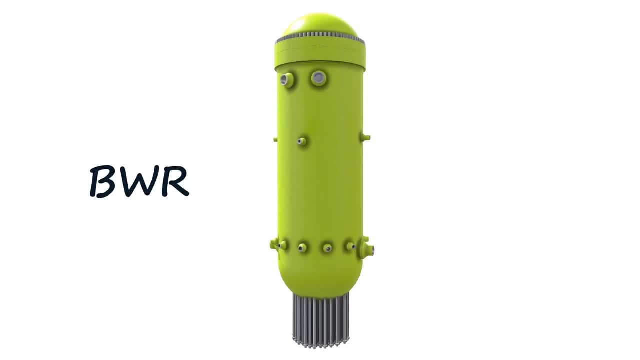 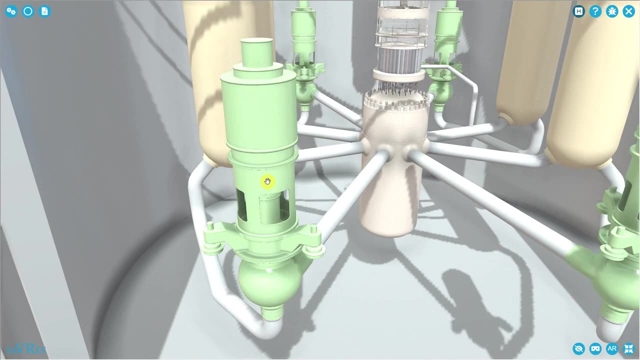 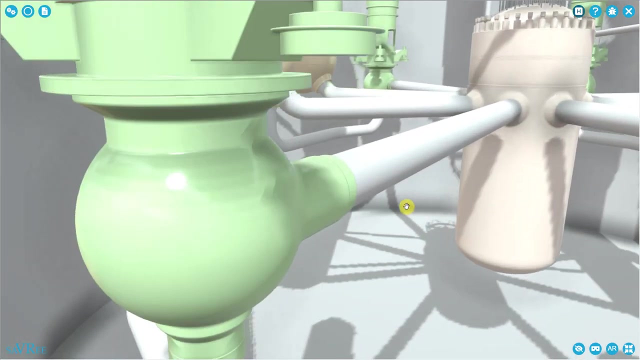 PWR and BWR, the two types of nuclear reactor that you're most likely to see. The reactor is our heat source. We've got reactor cooling pumps. Those are indicated in green here. They pump coolant through the reactor. What we'll do? we'll send the coolant in via this pipe here. 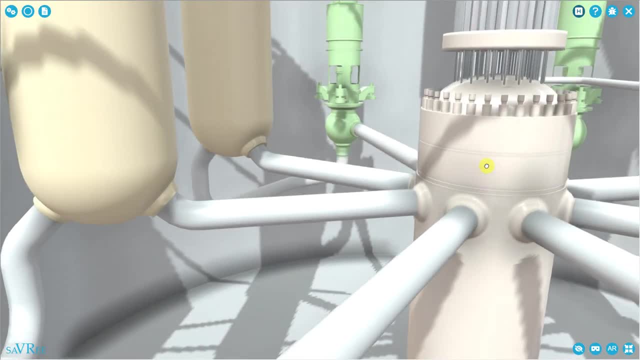 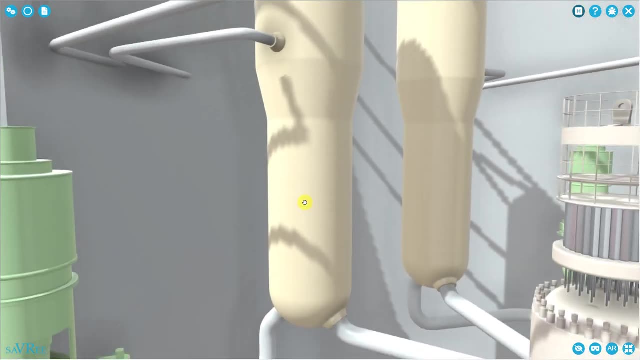 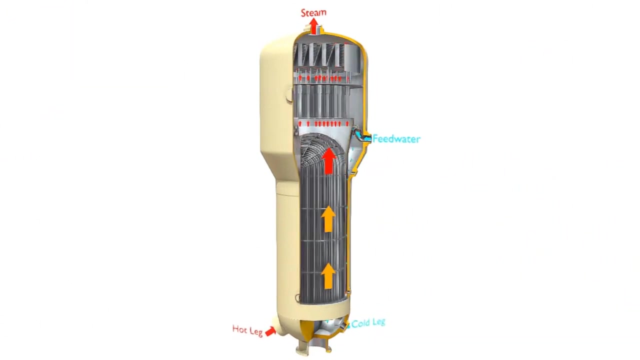 The coolant flows along here into the reactor, comes out, flows along here and then goes into a steam generator. The steam generator indicated by these cream-colored items are big heat exchangers. We pass the heat onto water within our steam generators. 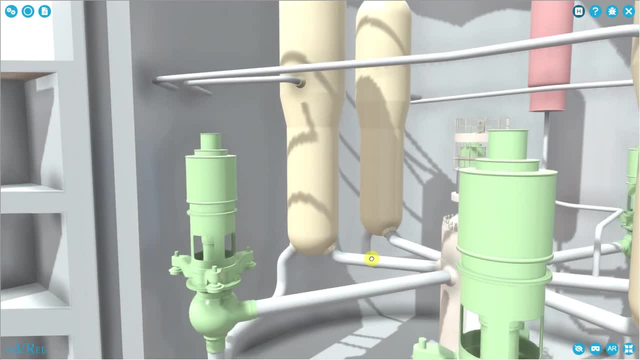 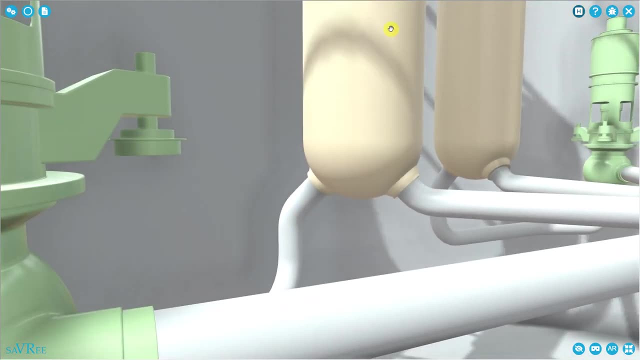 and that water will turn to steam. Before we have a look at that, though, let's just see where the coolant comes out. You can see the coolant comes out on this side, So it flows up into the steam generator. does a U? 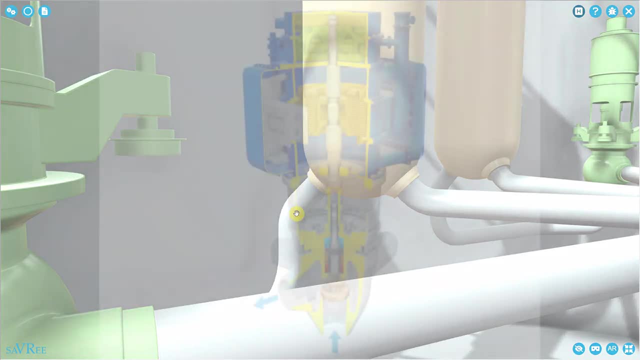 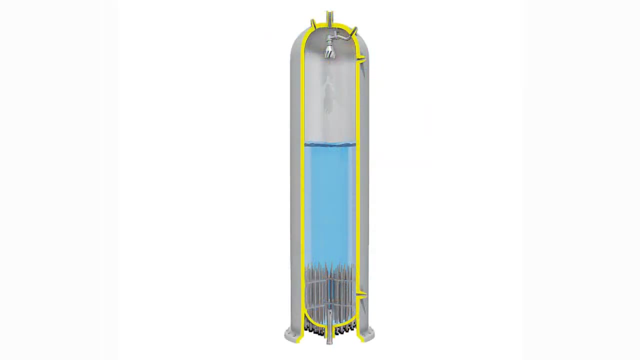 does a U-turn, flows back down again and comes out of the bottom. We've got a separate 3D model to show that. In fact, we've got separate 3D models for every one of these major components, So be sure to check those out in the 3D model library. 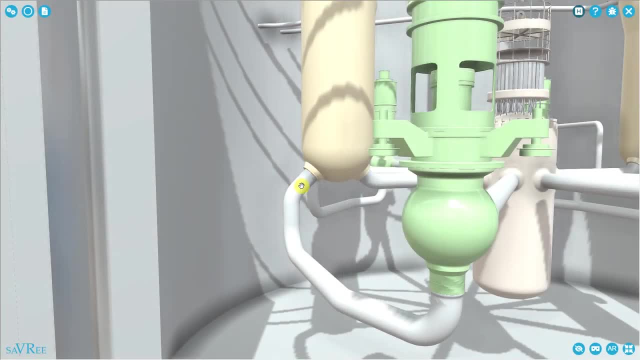 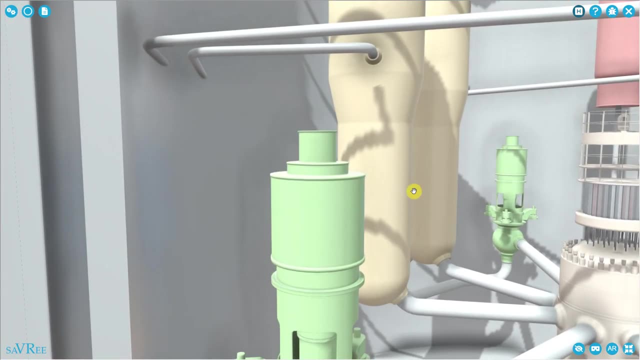 at savareecom, if you haven't already done so. The coolant flows along here, goes back into our reactor coolant pump and then the process begins again Within the steam generator. as I mentioned, we heat water which enters through this connection here. 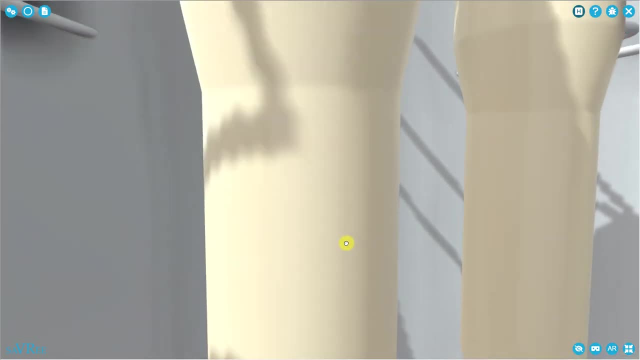 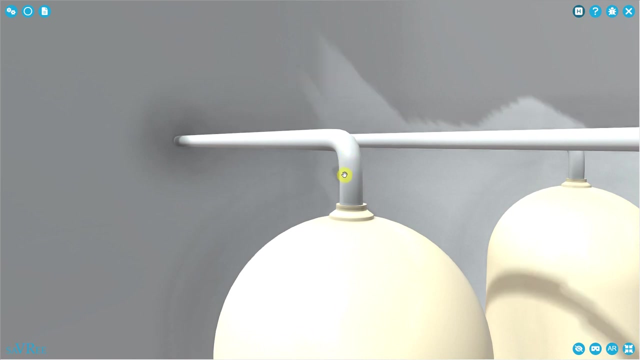 It actually goes down to the base of our steam generator and then goes back into the reactor And then flows back up again and we get steam coming out the top of the steam generator. Here is one steam outlet or steam discharge. Here is another. 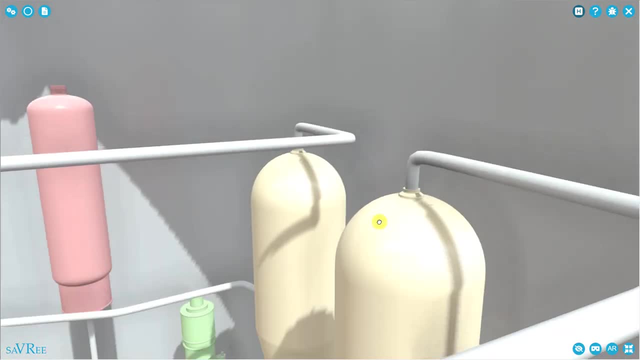 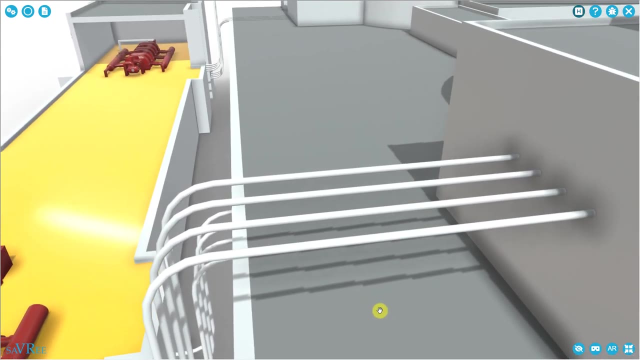 There's one at the top of each of our steam generators And we send that steam off to a steam turbine. See the four pipes coming out here. They may join all into one pipe. That would make a bit more sense- And the steam goes to a steam turbine over here. 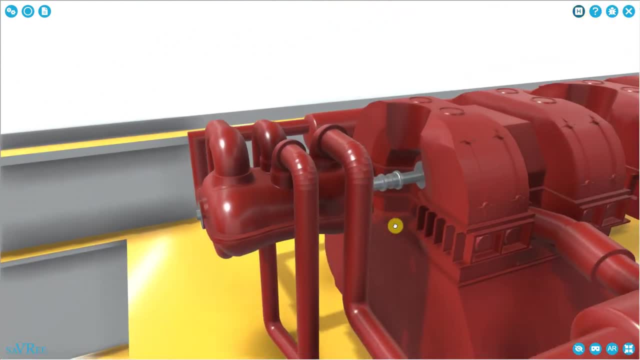 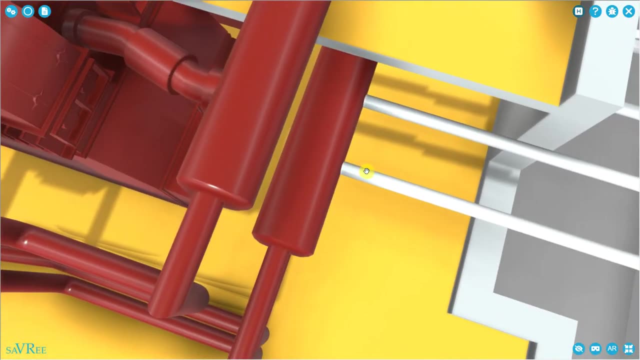 It will pass through a high-pressure steam turbine, maybe intermediate-pressure steam turbine, then through these low-pressure steam turbines. We've got three of those. You can actually see them if I zoom out. Here is one, Here is another, Here is another. 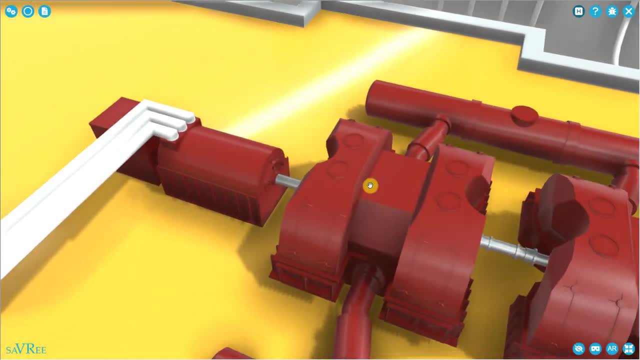 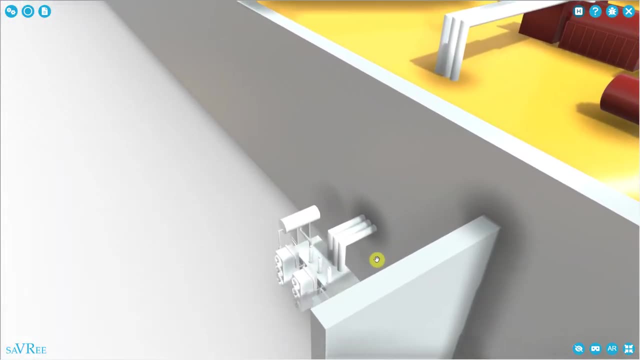 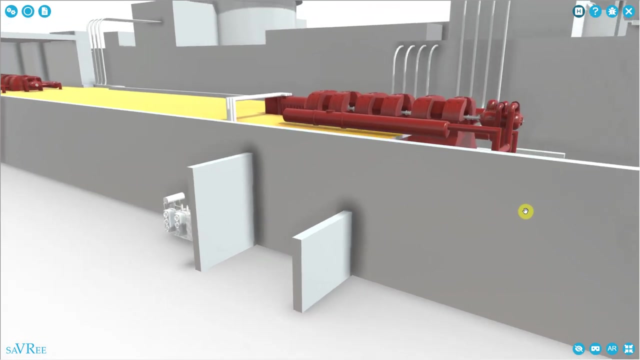 And all of those turbines connect to an electrical generator. That's this generator here, And then we generate electrical power and send it to an electrical transformer, this item over here. From there we can send the power to a substation and then to our power grid. 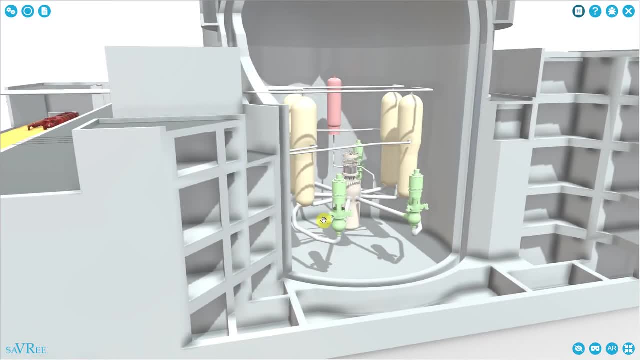 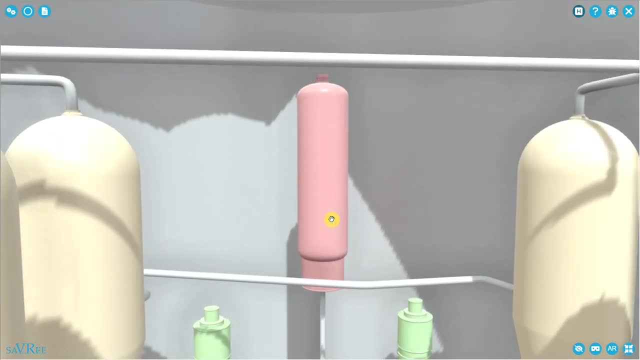 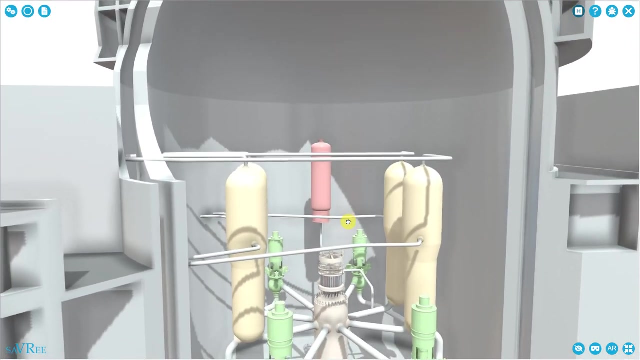 That's essentially how a pressurized water reactor nuclear power plant works. There are other components involved, such as a pressurizer- That's this pink item directly in the middle of the screen. now That has various functions within the system, but I don't think we need to discuss those right now. 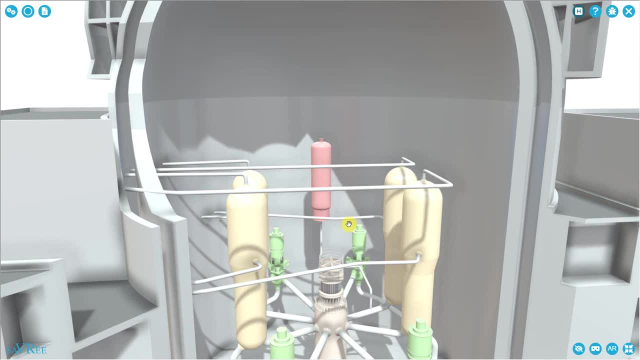 because this is an introduction video, just to give you a quick overview of how the power plant works, Irrespective of if you're looking for a power plant or if you're looking for an electrical power plant. irrespective of if you're looking for an electrical power plant. 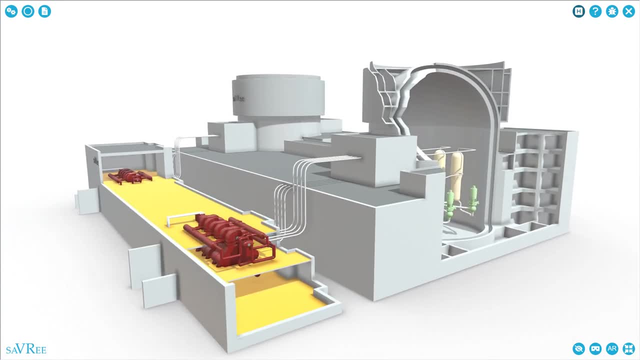 irrespective of if you're looking for an electrical power plant or if you're looking at a PWR or BWR, just keep in mind that reactors act as a heat source, and it's those heat sources that we need to turn water into steam.